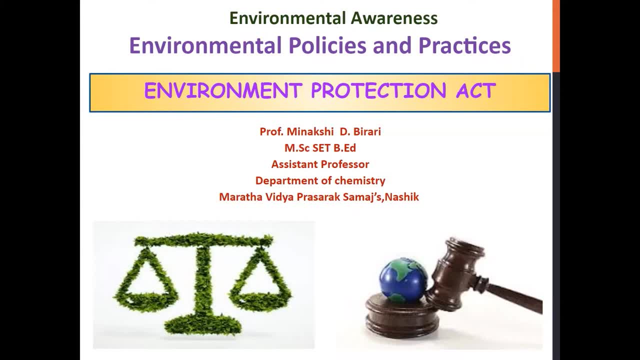 is threatened by a wide variety of human activities. So the main objective of Environment Protection Act is to provide the protection and improvement of environment and for matters connected therewith. The Act is one of the most comprehensive legislations with a pretext to protection and improvement. 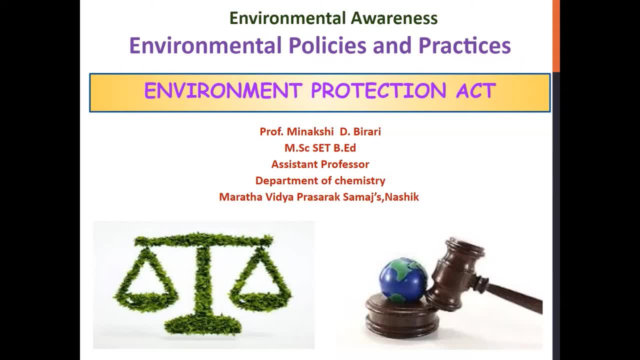 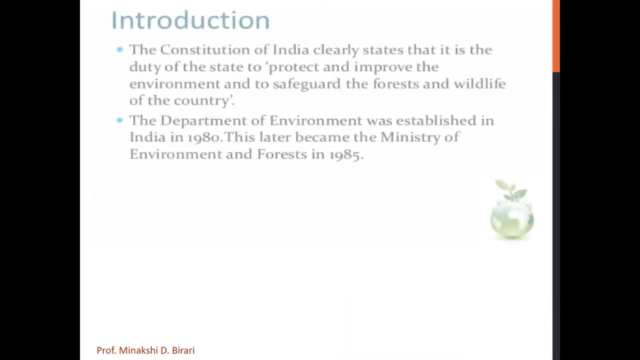 of the environment. The Environment Protection Act was enacted in the year 1986.. It was enacted with the main objective to provide the protection and improvement of the environment, The Environment and improvement of the environment. so let us see the different protection act related with air and also water. the Constitution of India clearly states: 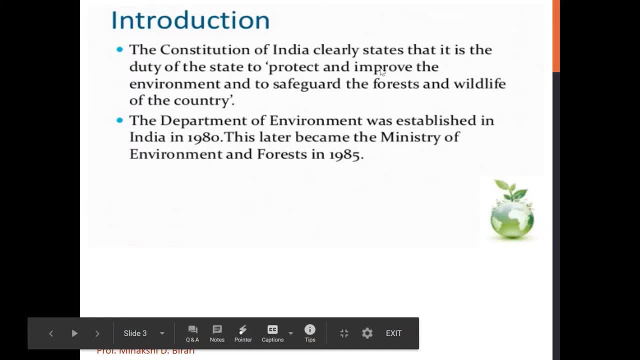 that it is the duty of the state to protect and improve the environment and to safeguard the forest and wildlife of the country. the Department of Environment was established in India in 1980. this letter became the Ministry of Environment and Forest in 1985. the Constitution of India also provides for: 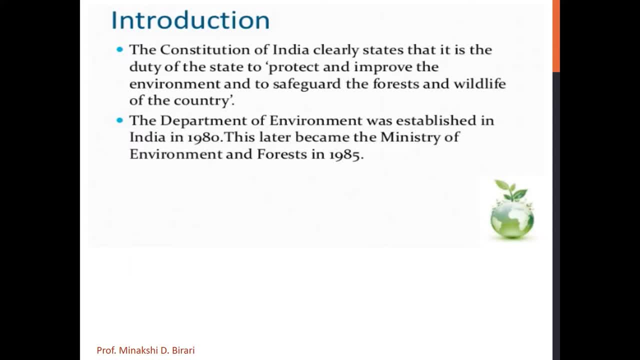 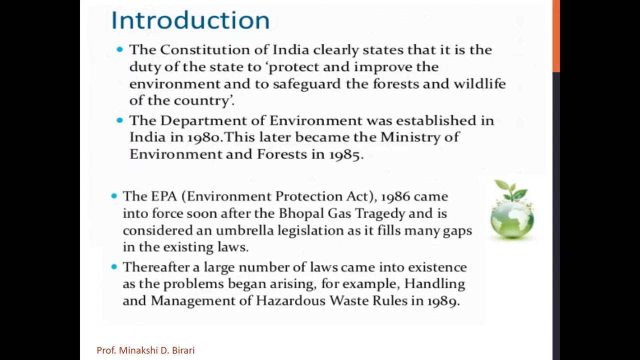 the protection of the environment. article 48 a of the Constitution specifies that the state shall endeavor to protect and improve the environment and to safeguard the forest and wildlife of the country. also, article 51a further provides that every citizen shall protect the environment. the Environment Protection Act 1986 came into force soon. 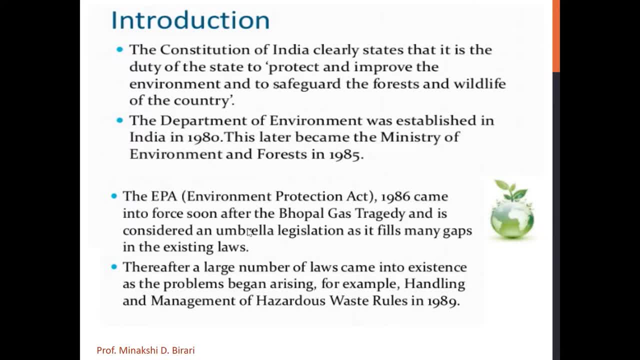 after the Bhopal gas tragedy, and it is considered an umbrella legislation as it fills many gaps in the existing laws. thereafter, a large number of laws came into existence. problems began arising, for example handling and management of hazardous waste rules in 1989. it is now generally accepted that environment is threatened by a wide variety of human activities. 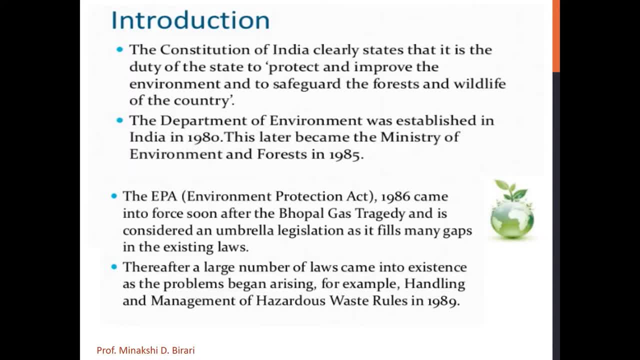 that ranges from the instinct, instinctive drive to reproduce its kind to the restless earth, of improving the standards of living, development and technological solutions to this end. the vast amount of waste, both that may be natural and chemical, that these advances produce. so, from time to time, various legislations have been enacted in india for this purpose. however, 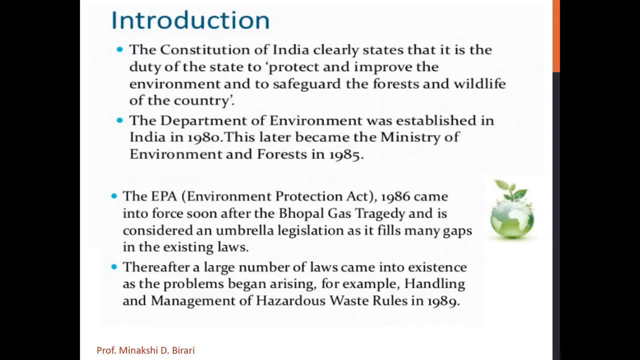 all legislations are prior to the 1986 act have been specific, relating to precise aspects of environmental pollution. however, the 1986 act was general legislation which is enacted under article 253 ie, legislation for giving effect to international agreements, so the first environmental protection act, that is. 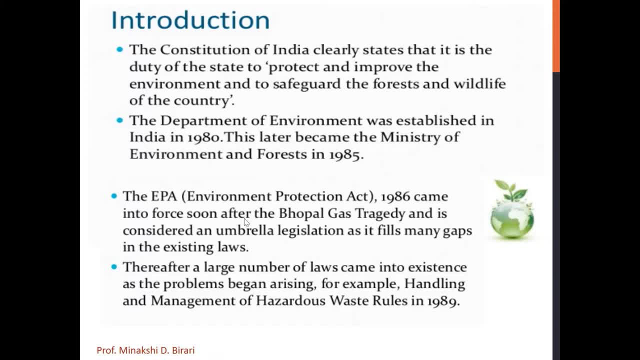 1986, came into force soon after the bhopal gas tragedy, and it is considered as the environmental protection act to which the law of family members were bestowed without any additional research was in place. as such became aware of the nature of environmental pollution. It is considered as an umbrella legislation as it fills many gaps in the existing laws. 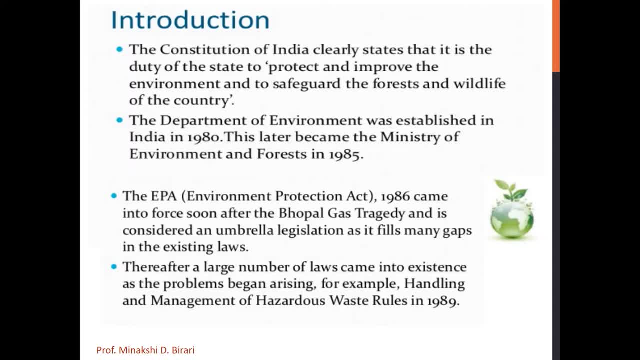 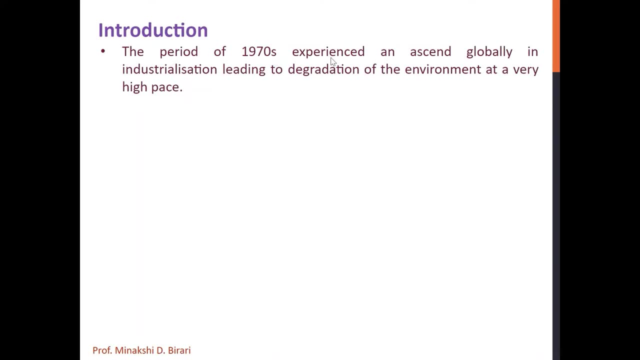 So in today's lecture we are going to discuss the Air Protection Act and umbrella legislation. So the period of 1970s experience and ascend globally in industrialization, leading to degradation of the environment at a very high pace, The need was filled for a combined effort towards environment conservation from all. 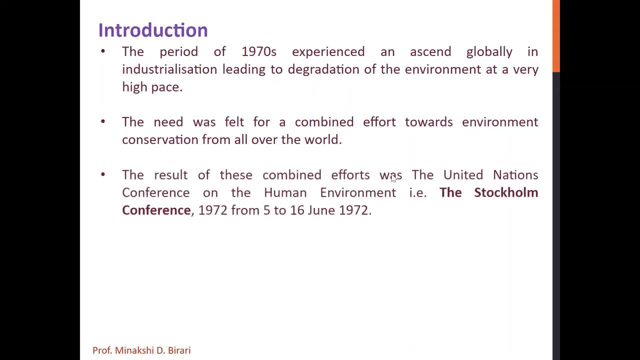 over the world. The result of these combined efforts was the United Nations conference on the human environment, that is, the Stockholm conference, which is in 1972, from 5 to 16 June 1972.. Then in India, Then in India, Then in India. 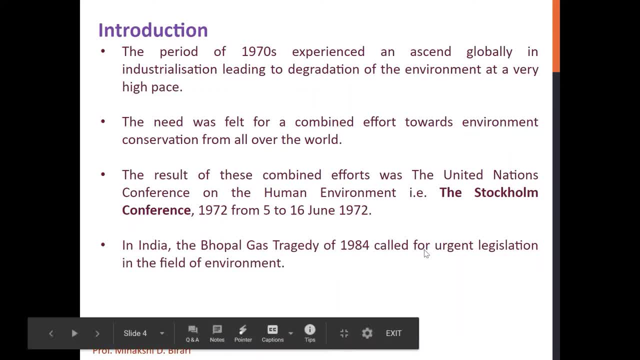 The Vopal Gas Tragedy of 1984 called for urgent legislation in the field of environment. In this background, the Parliament passed the Environment Protection Act 1986 and the Environment Protection Rules 1986.. India was a signatory to the Stockholm Conference of 1972, where the world community had resolved 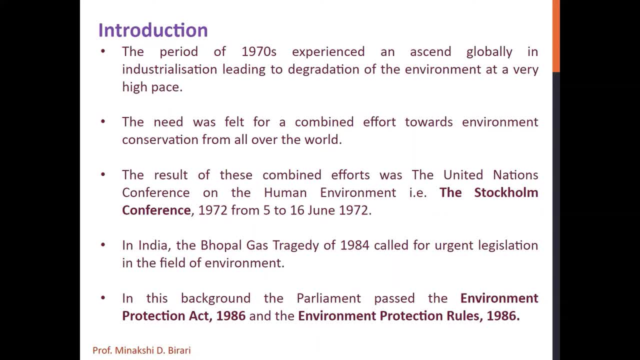 to protect and enhance the environment. While several legislations, such as the Water Prevention and Control of Pollution Act 1974 and the Air Prevention and Control of Pollution Act 1981 were enacted, after the conference the need for general legislation had become increasingly evident. 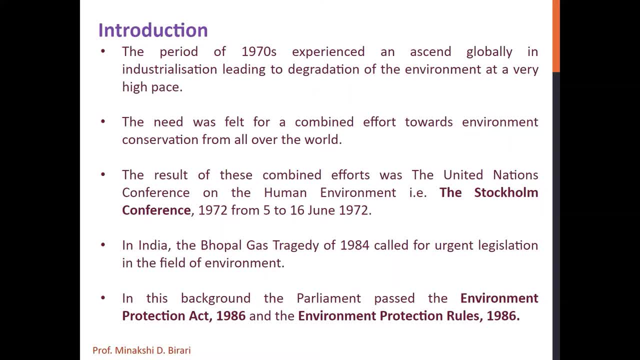 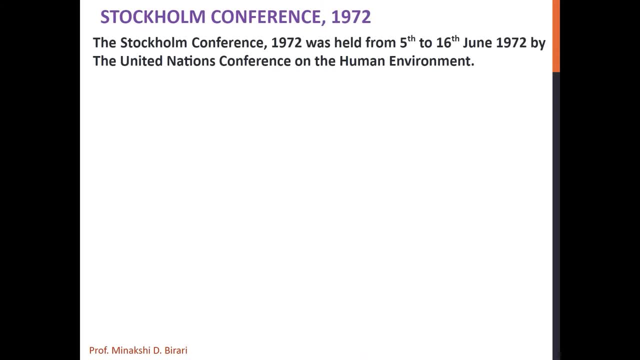 The EPA was enacted so as to overcome this deficiency. Mmmm, Please watch the video that publishes date and online. here have a few connection elements with the person who has adopted it. Stockholm conference at 1972.. The United Nations Conference on the Human Environment held in Stockholm in June 1972.. 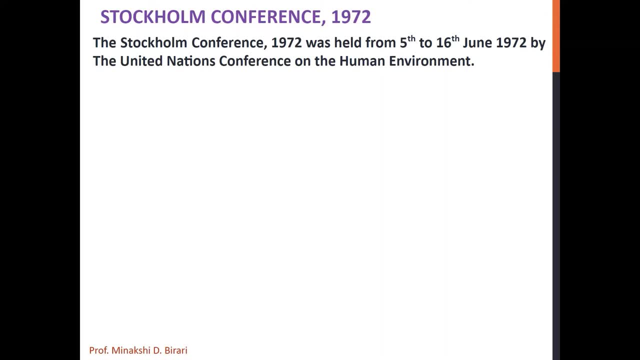 It was helped from June 5 to June 16, 1972 by United Nations Conference on the Human Environment. The focus of this conference was the state of the global environment. Its focus was health and medical arts and health policy concern. CNA conference was held in 1902. 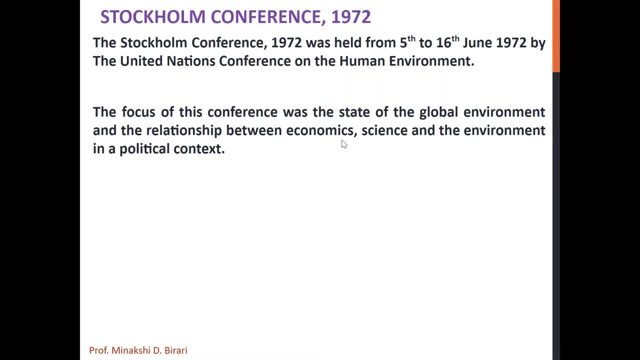 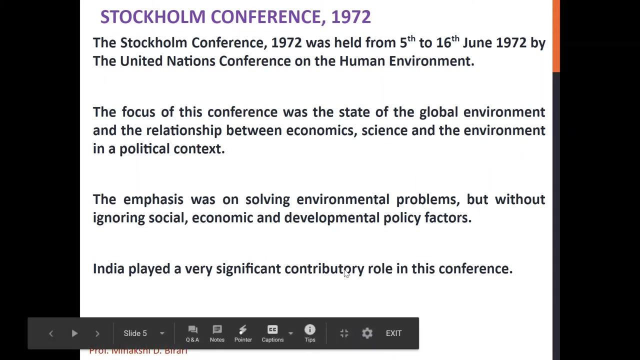 and the relationship between economics, science and the environment. in a political context, the emphasis was on solving environmental problems, but without ignoring social, economic and developmental policy factors. here India played a very significant contributory role in the conference. this conference laid the foundation of environmental legislation in India, so we should 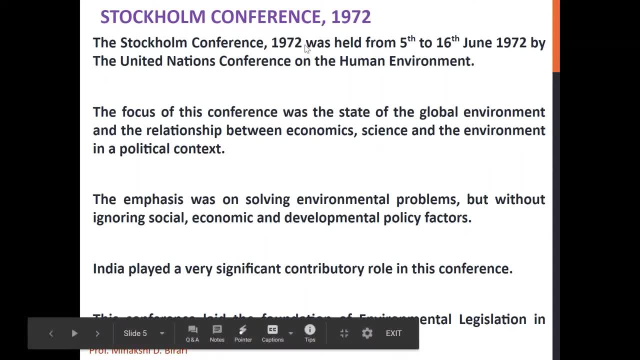 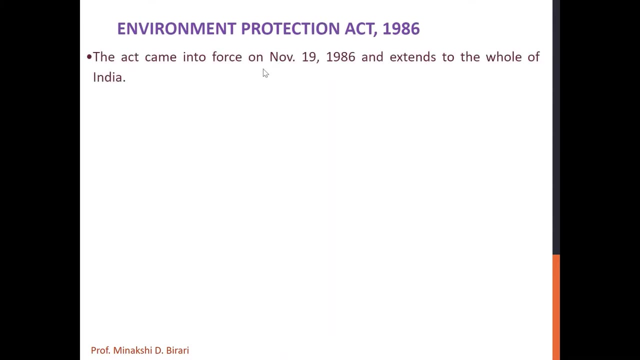 remember the Stockholm conference that is held in 72, from 5th June to 16th June 1972 by the United Nations Conference on the Human Environment: the Environment Protection Act. 1986: the act came into force. 2018: the Act came into force. the United Nationsだ was closed on October 15,. washermen and playgrounds. 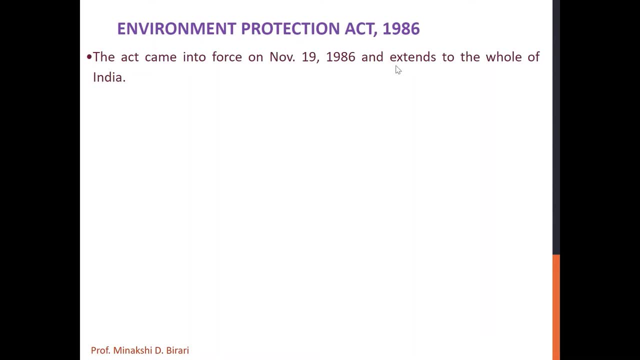 on November 19, 1986 and extends to the whole of India. The Act was passed to provide for the protection and improvement of environment and for matters connected therewith. The Act gives certain powers to the central government to take measures for the purpose. 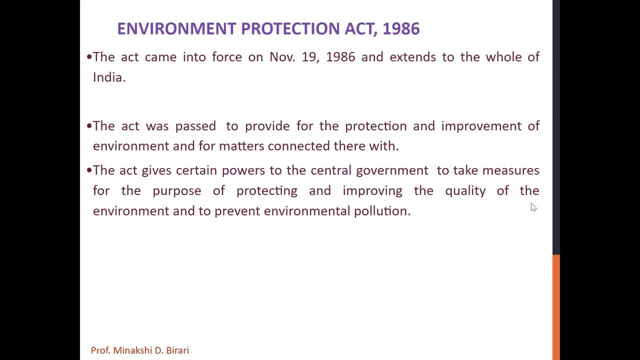 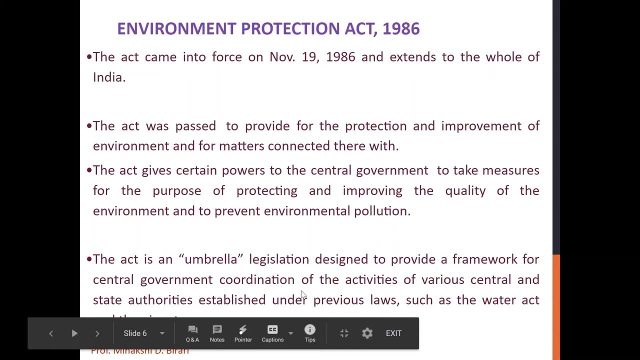 of protecting and improving the quality of the environment and to prevent environmental pollution. The Act is an umbrella legislation designed to provide a framework for central government coordination of the activities of various central and state authorities established under previous laws, such as the Water Act and the Air Act. 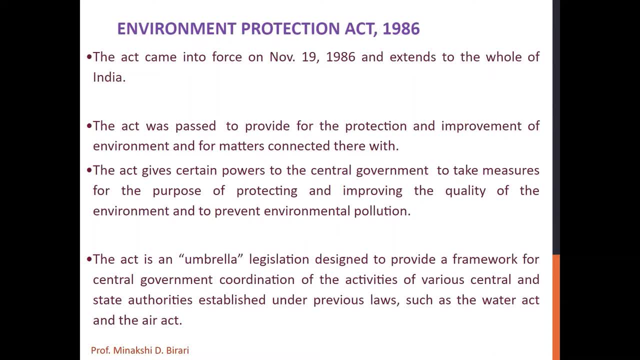 The Environment Protection Act is applicable to the whole of India. In fact, it is applicable to the whole of India. It came into force on November 19, 1986.. According to Section 2,, the EPA Environment Protection Act gives the definition of environment. 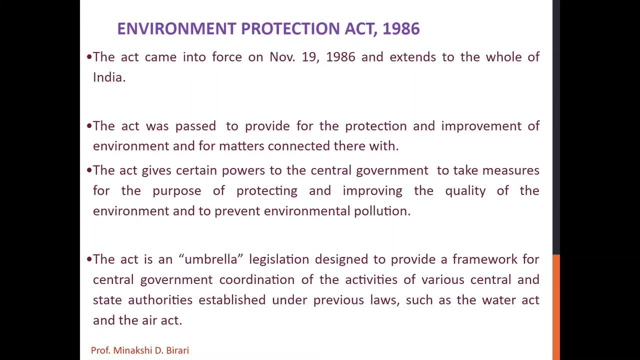 that includes water, air and land and the interrelationship that exists among and between water, air and land and human beings. This includes living creatures, plants, microorganisms and property. So this definition is not exhaustive, but an inclusive one. Also, environmental pollutants: that means any solid, liquid or gaseous substances that 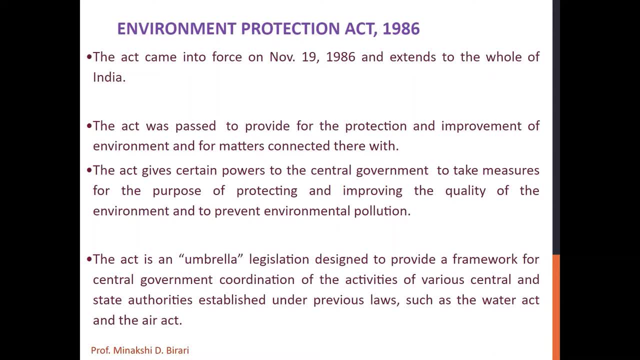 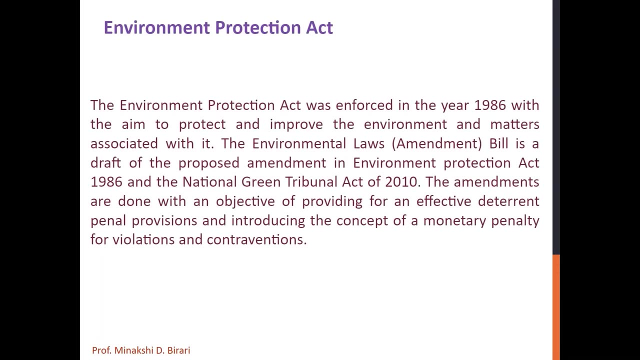 are present in such a concentration as may be, or tend to be, injurious to environment. So that may be, then, according to Section 2 of the EPA. Thank you. The Environmental Protection Act was enforced in the year 1986 with the aim to protect and. 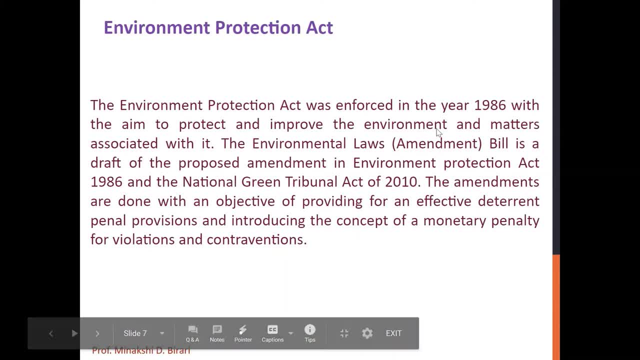 to improve the environment and the matters associated with it. The Environmental Laws Bill is a draft of the proposed Amendment in Environment Protection Act 1986 and National Green Tribunal Act of 2010.. Thank you. The amendments are done with an objective of providing for an effective deterrent penal provisions and introducing the concept of a monetary penalty for violations and contraventions. 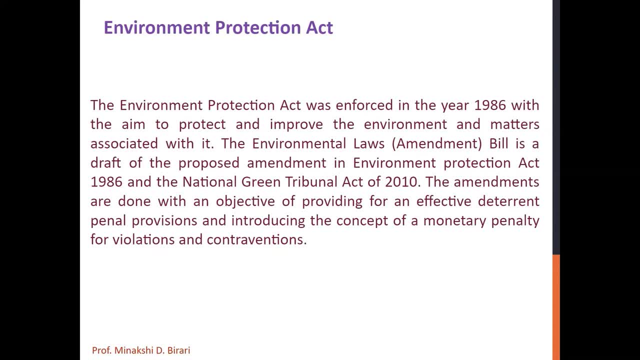 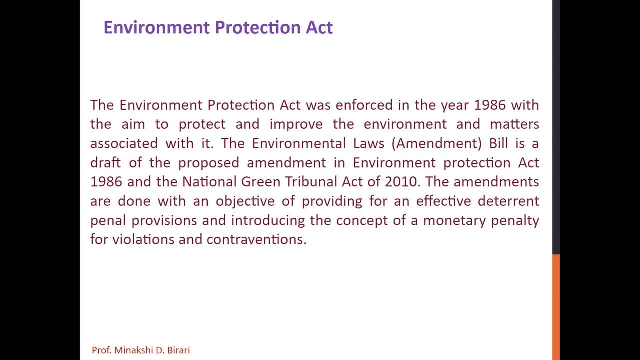 race as a whole. so the environment protection act that was enforced in the year 1986 and the aim of the environment protection act that is, to protect and improve the environment and the matters associated with it. and what is the environmental law? the environmental law? it consists of a wide 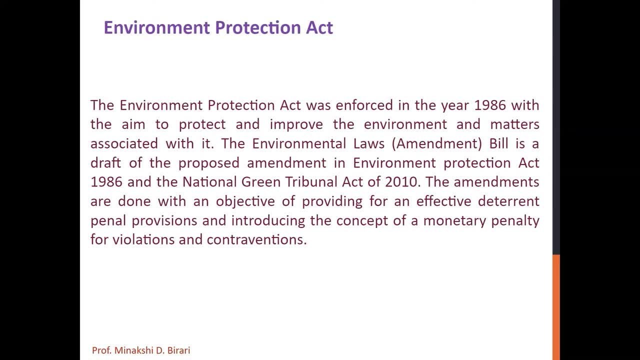 variety of legislation, enactments and provisions that are chiefly concerned with the regulation of human activity concerning our natural environment and its various interconnected ecosystems. while everything that is encompassed in environmental law may not directly intersect with each other, they all act as a safeguards in preventing environmental damage and ensuring 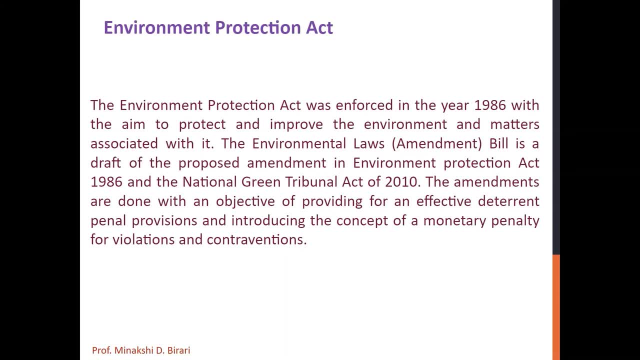 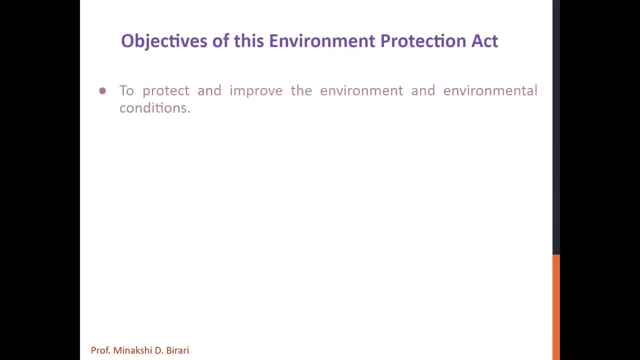 a safe and safe, sustainable, effective management of the environment and its multiple ecosystem. So the main objective of Environment Protection Act is to provide the protection and improvement of environment and for matters connected therewith. So what are the objectives of this Environment Protection Act? To protect and improve the environment and environmental conditions. to implement the 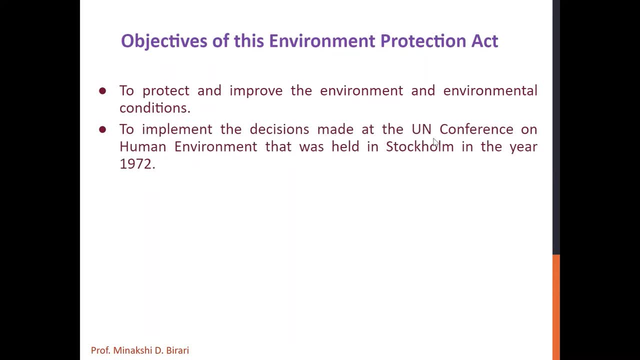 decisions made at the UN conference- United Nations Conference on Human Environment that was held in Stockholm in the year 1972,. to take strict actions against all those who harm the environment. to enforce laws on the environment protection in the areas that are not in the environment. 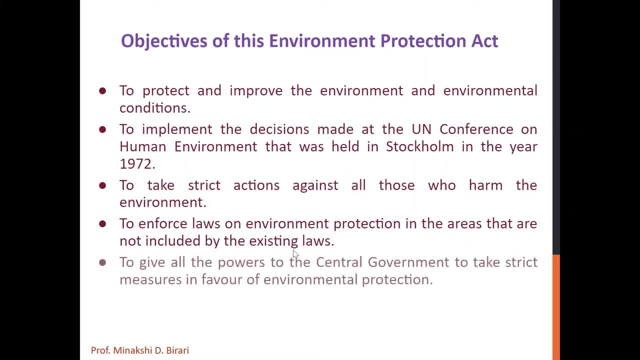 Included by the existing laws and to give all the powers to the central government to take strict measures in favor of environmental protection. The Constitution of India also provides for the protection of the environment. Already I have explained that Article 48 of the Constitution specifies that the state 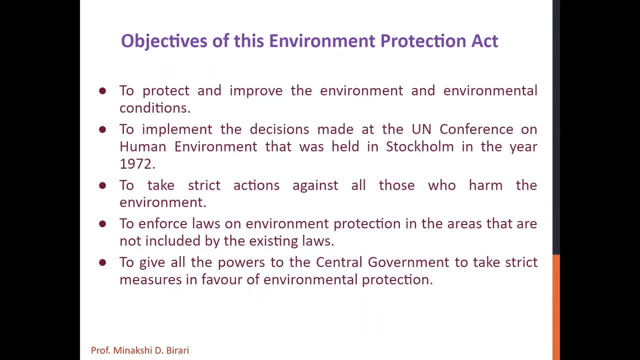 shall endure, to protect and improve the environment and to safeguard the environment. This law also provides for the protection of the environment and the forests and also the wildlife of the country. Also, Article 51a further provides that every citizen shall protect the environment. 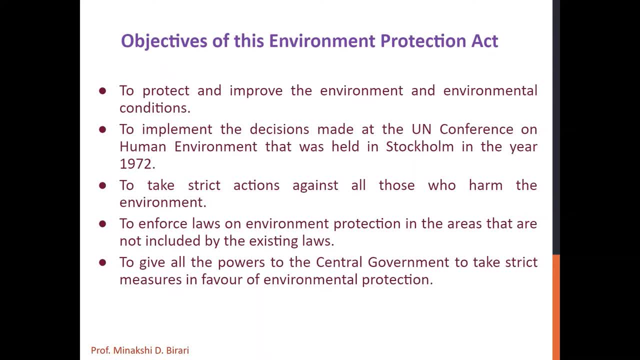 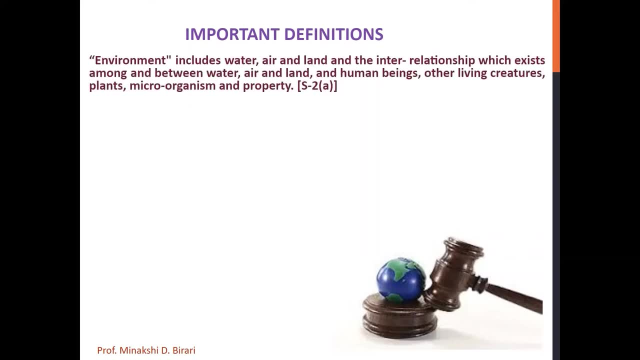 So these are the objectives of this Environment Protection Act. Now, what are the definitions which are according to Environment Protection Act 1986?? So first one, environment, That is, it includes water, water and soil. So these are the objectives of this Environment Protection Act. 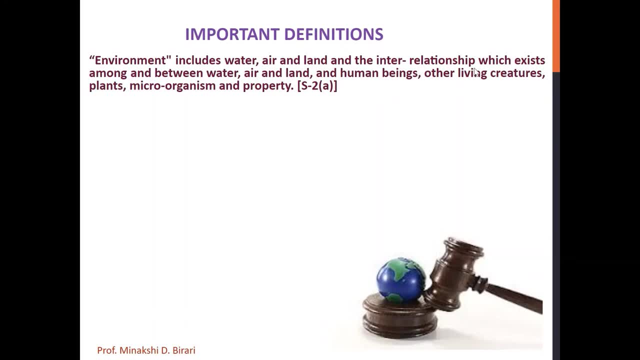 air and land and the interrelationship which exists among and between water, air and land and human beings, other living creatures, plants, microorganisms and property. so that is, according to section 2a, also environmental pollutant. that means any solid, liquid or gaseous substances present in such a concentration as may be or tend to be injurious or 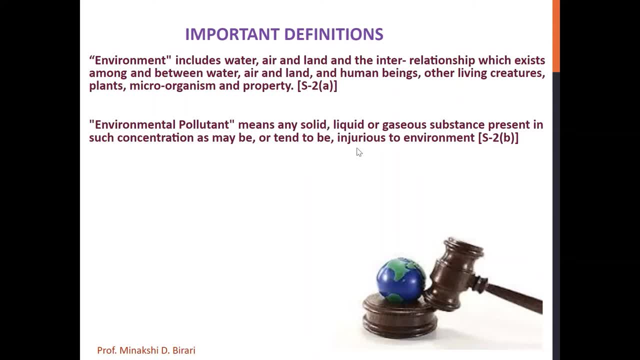 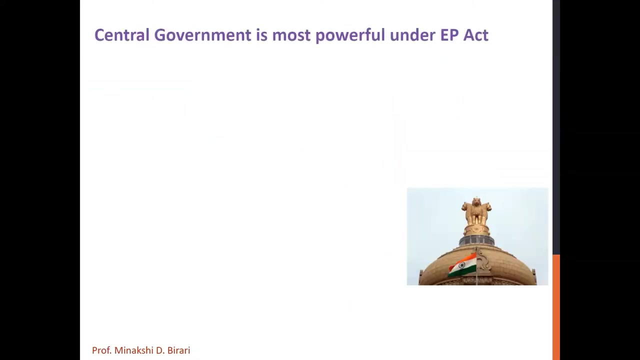 injurious to the environment. then third one: environmental pollution. so what is the definition of this? that means the presence in the environment of any environmental pollutant that causes the pollution. environmental pollution according to section 2c. so these are the important points and important definitions. next to that, central government is most powerful under ep act. 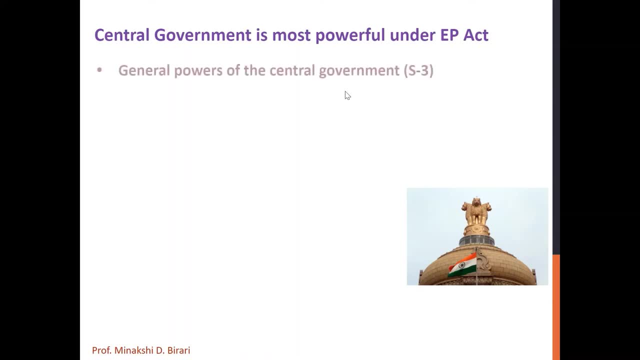 environmental pollution act. the general powers of the central government is three that are: take all necessary measures for environmental protection. they can coordinate the actions of the state governments, lay down standards of environment quality and pollutants, execute nationwide programs. also restriction of areas for industries, etc. inspecting industrial premises. preparation of manuals, codes, guides. 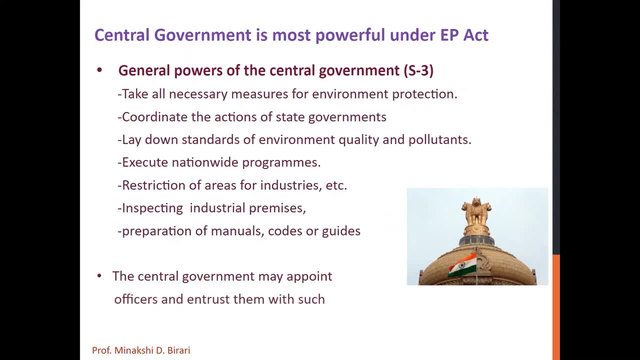 The central government may appoint officers and entrust them with such powers and functions as it may deem fit. So these are the general powers of central government. Central government is most powerful under EP Act, So we should remember what are the general powers of central government. 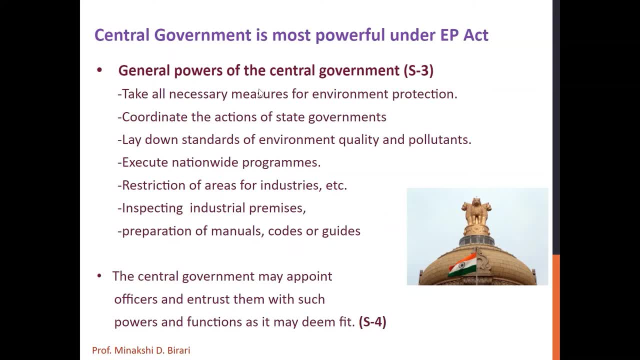 They can take all necessary measures for environment protection, coordinate the actions of state government, Also lay down standards of environment quality and pollutants. They can execute nationwide programs, also restrict of areas for industries, inspect industrial premises and also prepare the manuals or codes or guides. 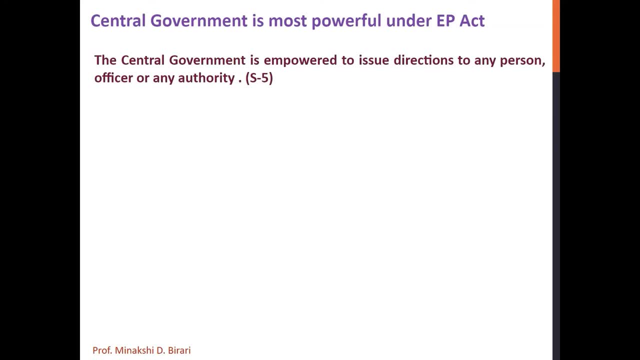 The central government is empowered to issue directions to any person, officer or government officer or any authority. So closer direction that means with power to disconnect electricity and water supply. The central government is empowered to make rules to regulate environmental pollution on the following matters: 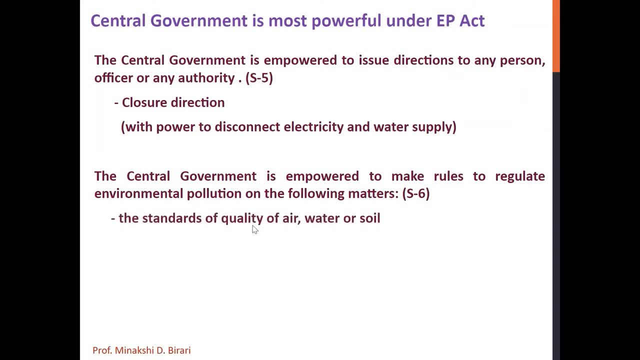 So what are that? First, the standards of quality of air, water or soil, Also the maximum allowable limits of pollutants, The procedures For the handling of hazardous substances, The prohibition and restriction on the location of industries And the procedures and safeguards for the prevention of accidents. 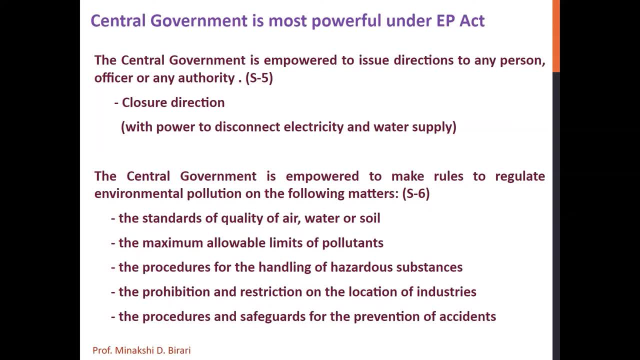 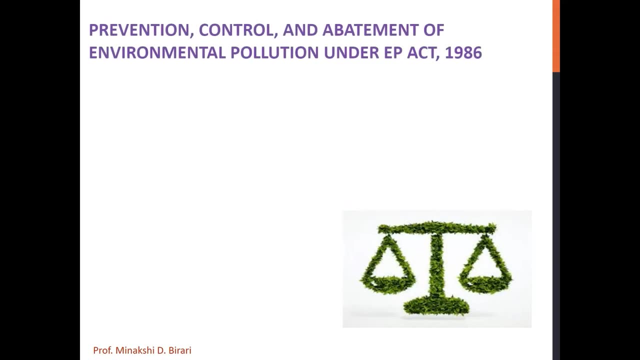 So to regulate the environmental pollution, these are the different matters which can be empowered by the central government. Now let's talk about the environmental pollution. So, the environmental pollution, The environmental pollution. Now, what are the prevention or control measures to reduce the environmental pollution under 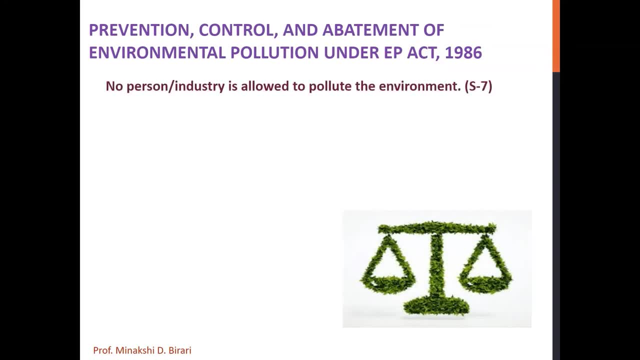 EP Act 1986.. First thing, that no person or industry is allowed to pollute the environment. Then procedures and processes are laid down to control pollution Monitoring authority can carry out inspections. Power to take samples as per the prescribed procedures. Samples are also tested in environmental laboratories. 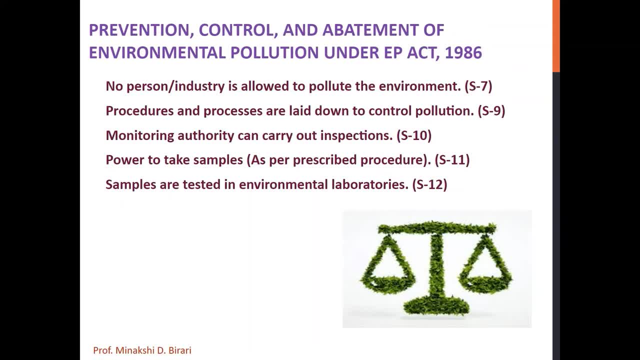 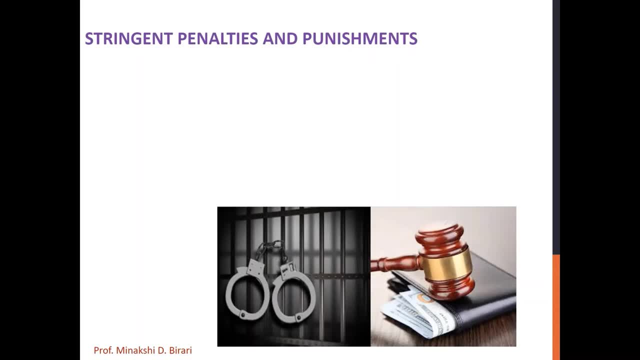 Then there are some state penalties and also some punishments: Whoever contravenes the provisions of the act. maximum punishment up to 7 years and penalty up to Rs.100000 or Rs.5000 per day for continued offenses. The same applies to water. 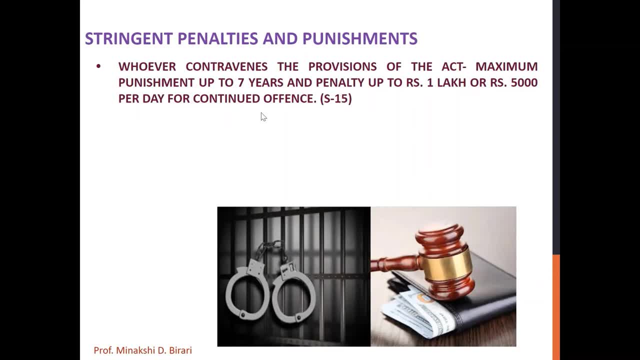 The same applies to the water, The same applies to the air, The same applies to the water, The same applies to the chemicals. For defaulter companies or body corporates, directors or partners are prosecuted. This act is also applicable to government departments and HOD prosecuted. 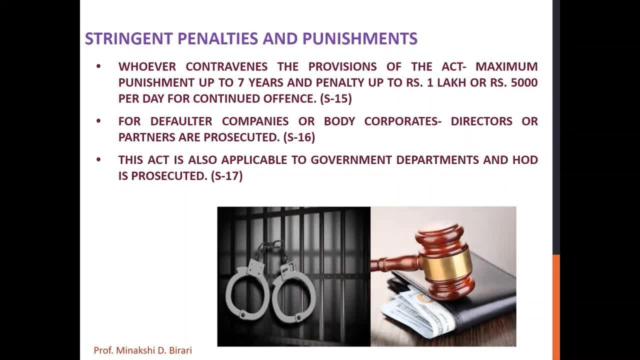 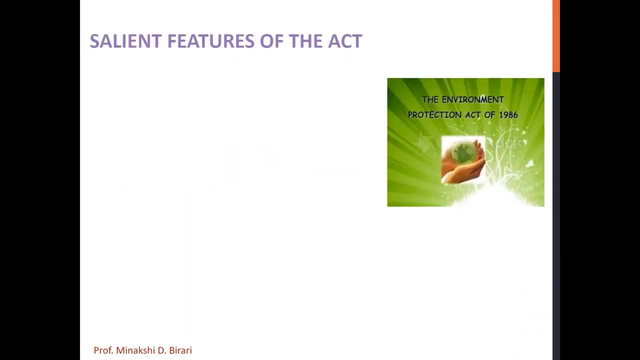 So what are the penalties or punishment: Maximum punishment up to 7 years and penalty up to Rs 1 lakh or Rs 5000 per day for continued offence. Silent features of the act. So what are that? First one: this act deals with the criminal jurisdiction and central government is most powerful. 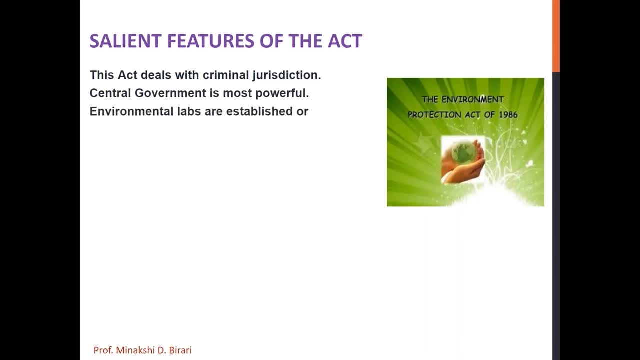 Environmental labs are established or authorized by central Central government, state government, CPCB or state PCB. Standards are laid down by central government, standard government, CPCB or state PCB Person having highest authority is prosecuted and the hazardous waste are defined and special procedure is laid down for that. 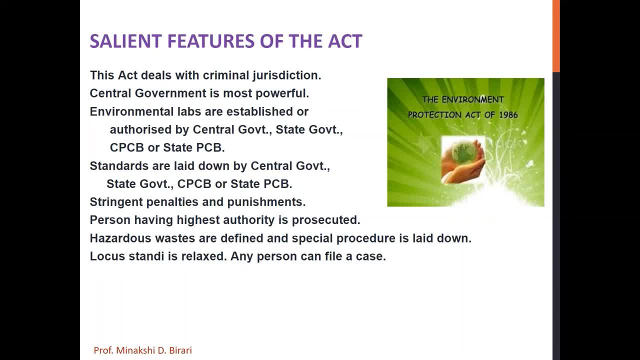 Local standing is relaxed. Any person can file a case. This act is also applicable to government department, and that is, this is an umbrella legislation. So these are the silent features of the act. Now, what is umbrella legislation? There are several rules laid down under the EP Act. 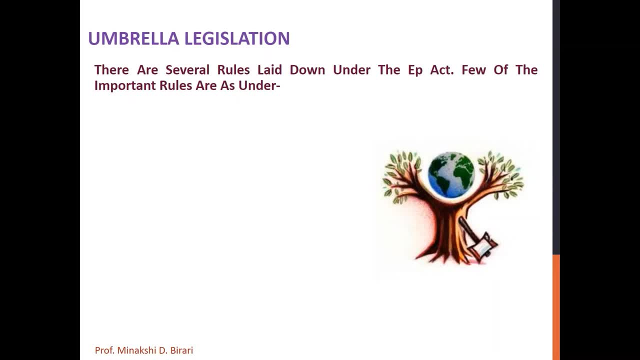 Few of the important rules are as under First: Environmental Protection Rules 1986.. Hazardous Waste Rules 1986.. Biomedical Waste Rules 1998.. Biomedical Waste Rules 1998.. Municipal Solid Waste Rules 2000.. Noise Pollution Rules 2000.. 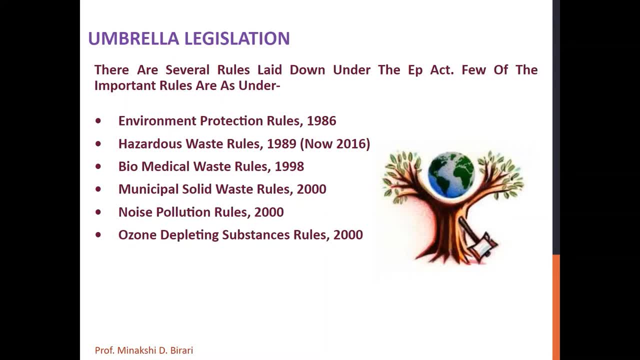 Ozone Depleting Substances: Rules 2000.. Also, Battery Waste Rules 2001.. Plastic Waste: Rules 2011.. Electronic Waste: Rules 2011.. So there are several rules laid down under the EP Act And Few of the important rules are under umbrella legislation. 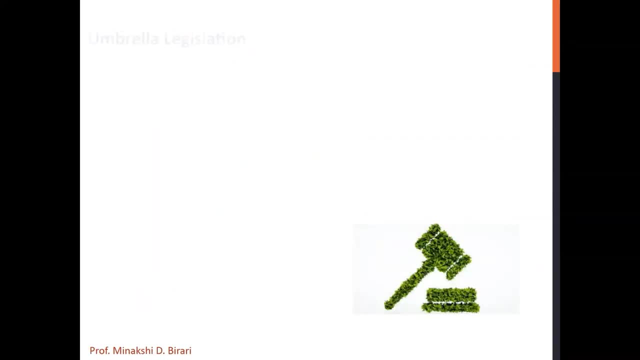 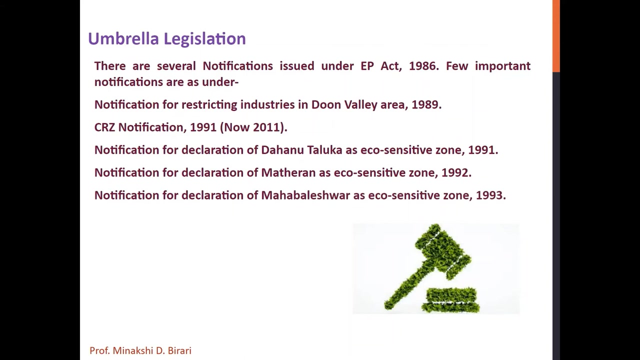 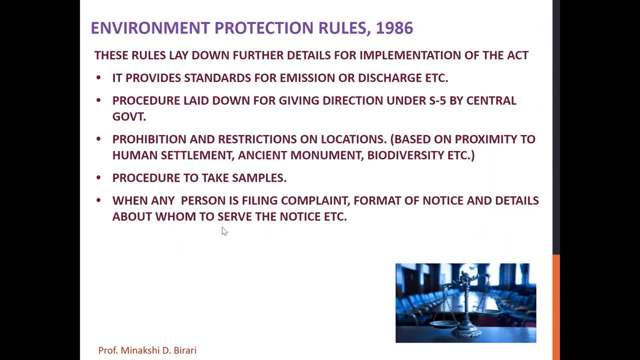 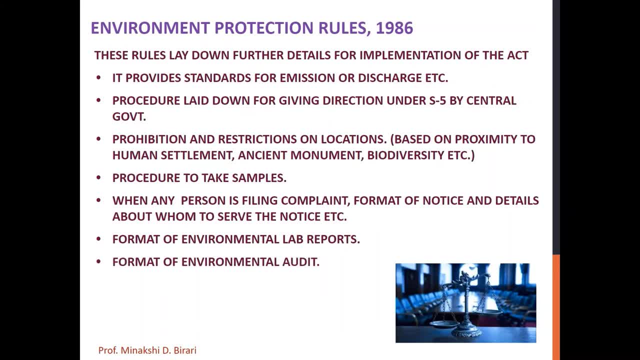 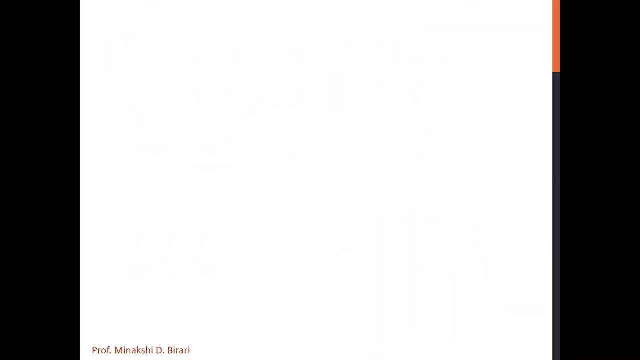 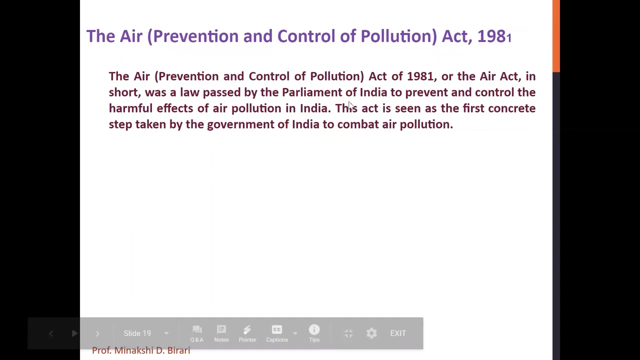 environmental audit. so these are the rules lay down further details for implementation of the act 1986. now let us see the air prevention, control of pollution act 1981. the air prevention and control of pollution act 1981, or the air act in short, was a law passed by the Parliament of India to prevent and 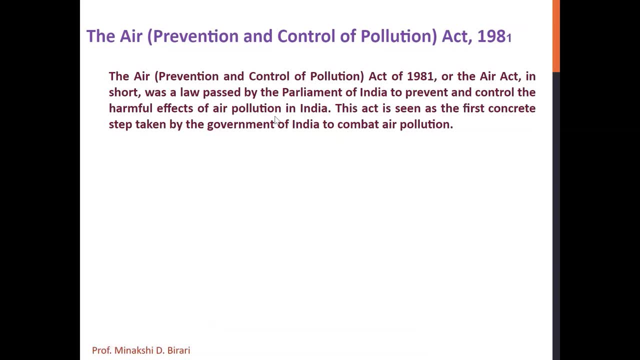 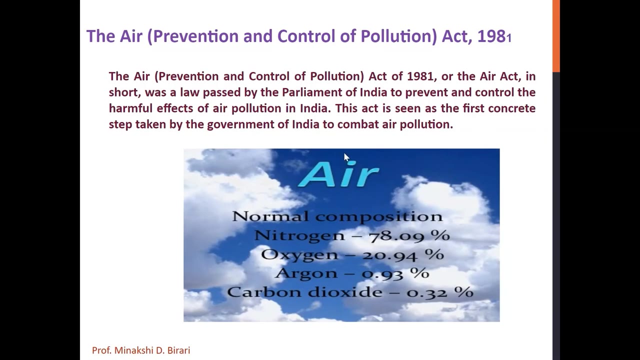 control the harmful effects of air pollution in India. this act is seen as the first concrete step taken by the government of India to combat air pollution. we know that air having the composition- normal composition, that is, it contains nitrogen about 78%, oxygen 20.94%, argon 0.93% and carbon dioxide 0.32%. so the 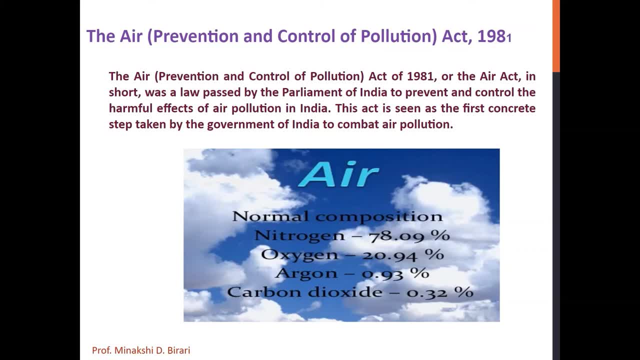 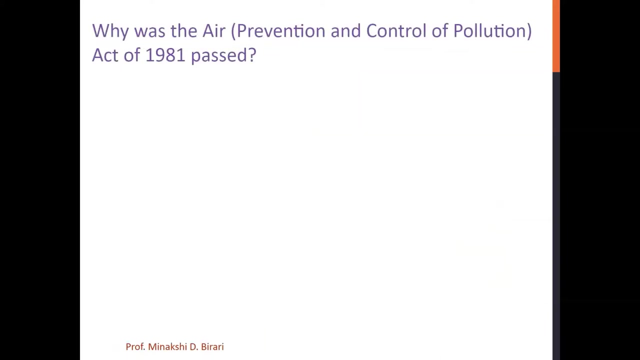 air act in short, was a law which is passed by the Parliament of India to prevent and control the harmful effect of air pollution in India, and this act is seen as the first concrete step taken by the government of India. why was the air act of 1981 passed? so the effect of climate change caused by 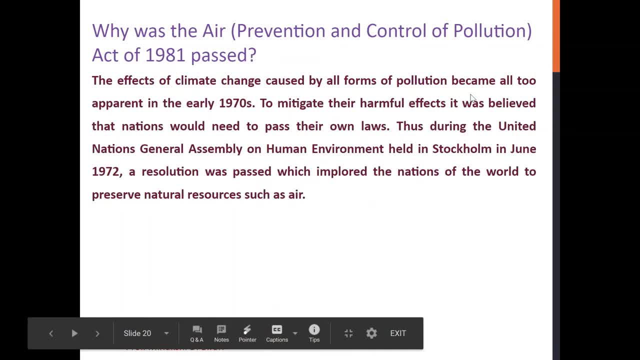 all forms of pollution became all too apparent in the early 1970s. to mitigate their harmful effects, it was believed that nations would need to pass their own laws. thus, during the United Nations General Assembly on human environment, which is held in Stockholm, in June 1972, a resolution was passed. 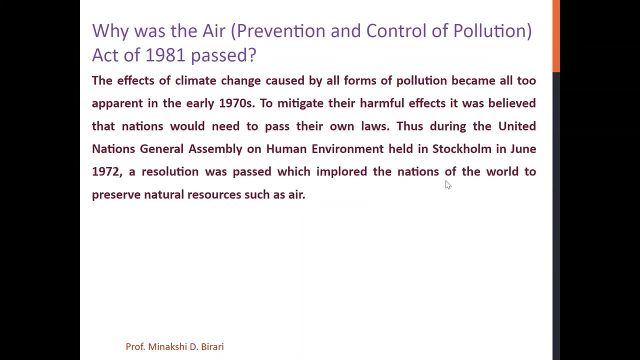 which implored the nations of the world to preserve natural resources such as air so the India itself had issues regarding air pollution against theредs in the Scottish environment which I am going to cover in this video. the very method of air pollution as 구조 � Wanzburg named this act ice and then to theылis from the United Nations General Assembly in May 1971. it was coded as today: in the United Nations General Assembly on Human Environment, which is held in Stockholm in June 1972, a resolution was passed which implore the nations: 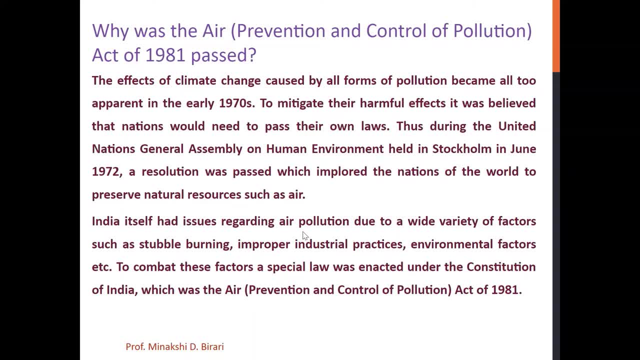 of the world to preserve natural resources such as air according to nature. It came to some reference. government of the United Nations General Assembly of China. pollution due to a wide variety of factors, such as stubble burning, improper industrial practices, environmental factors, etc. To combat these factors, a special law was enacted under 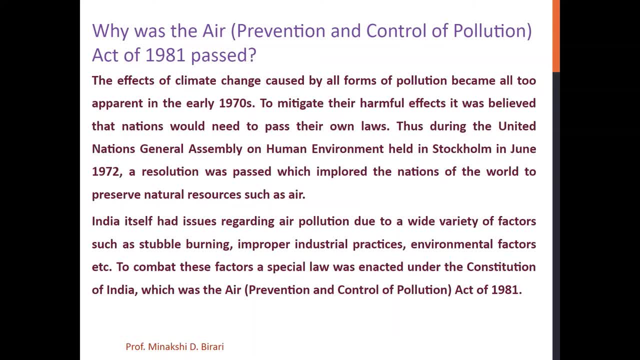 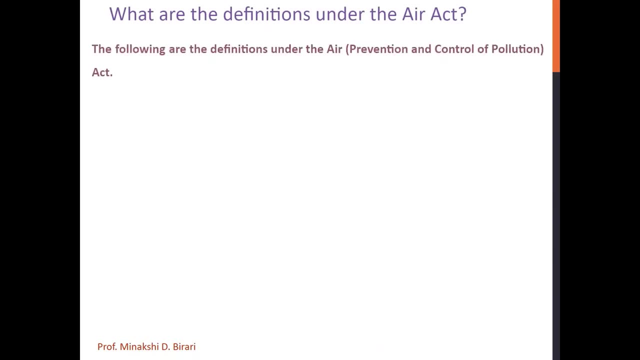 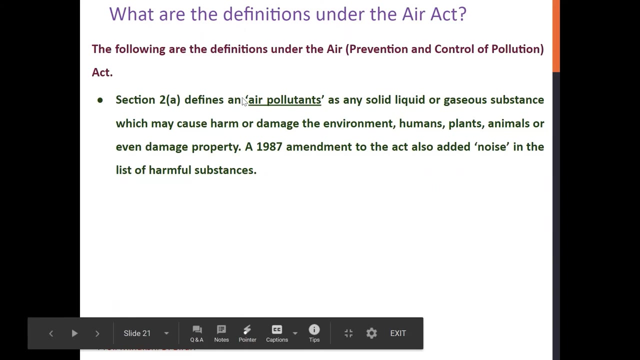 the Constitution of India, which was the Air Prevention and Control of Pollution Act of 1981. What are the definitions under the Air Act? There are two definitions under the Air Act. According to Section 2,, it defines an air pollutant which are any solid liquid or. 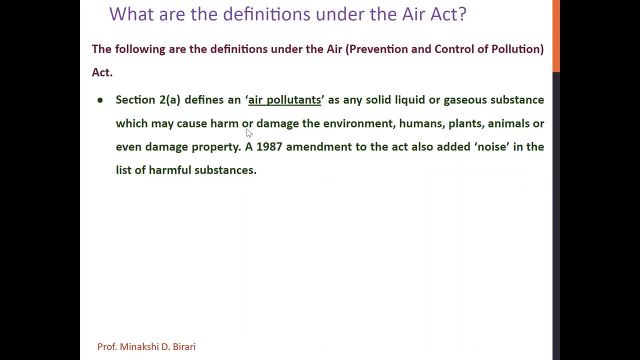 gases which may cause harm or damage to the environment based on its type. The air pollutes are those things which are damaged or destroyed in the form of neighborhoods, humans, plants, animals or even damage property. A 1987 amendment to the Act also added noise. 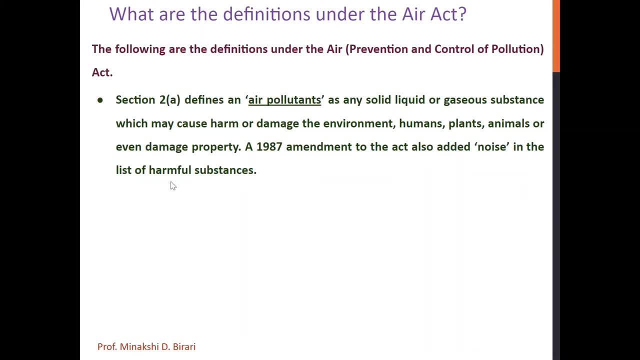 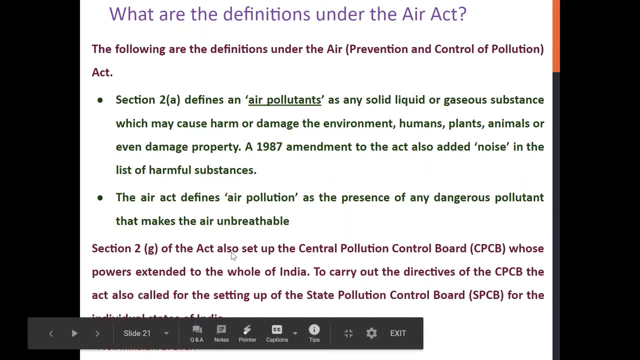 in the list of harmful substances. The Air Act defines air pollution as the presence of any dangerous pollutant that makes the air unbreathable. Section 2 of the Act also set up the Central Pollution Control Board, whose powers extended to the whole of India to carry out the directives of the CPCB. The Act also called for the setting 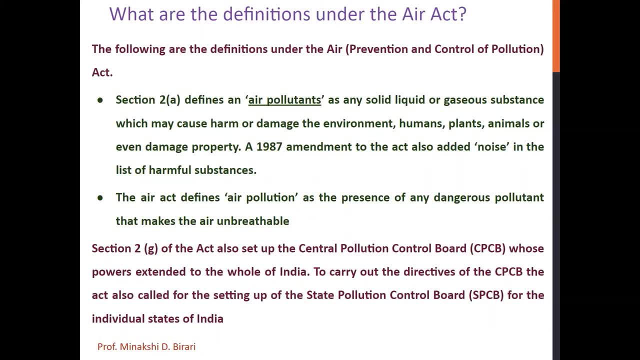 up of the State Pollution Control Board for the individual states of India. Air Act refers to the measures adopted to maintain safe air standards, ie enforcing rules which allow air pollution control to be maintained within the state Air Act also, and regulations after determining what is the safe level of emission in terms 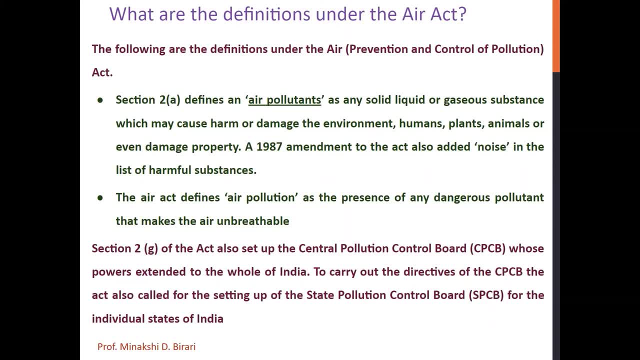 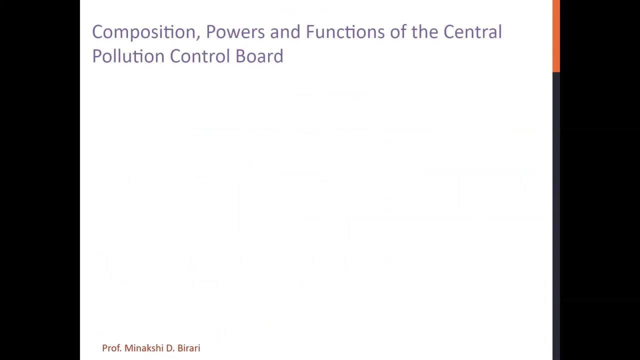 of motor vehicles, industrial emissions and common everyday uses. the most common example of this is the emission test and regular cyclic vehicle safety test. so the air act. it is helpful in reducing air pollution and maintaining air quality. now what is the composition, powers and functions of the Central? 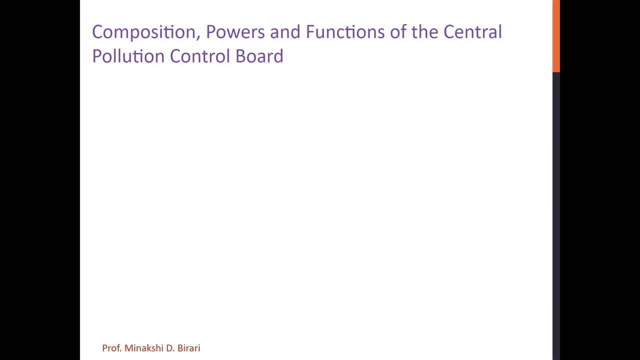 Pollution Control Board, CPCB. the CPCB would have a chairman with crucial knowledge regarding environmental protection. he or she would be aided by secretary appointed by the central government. in addition, five more members would be nominated by the central government. the functions of the CPCB would be the following. 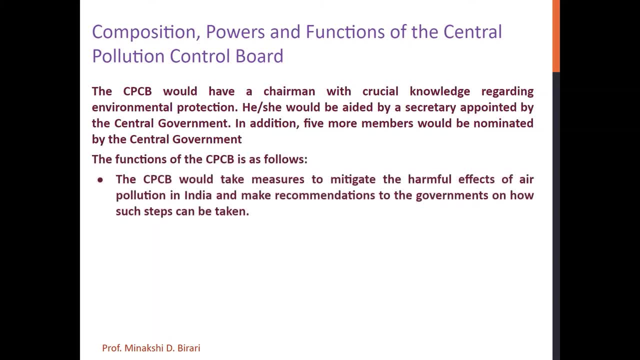 CPCB are that take measures to mitigate the harmful effects of air pollution in India and make recommendations to the governments on how such steps can be taken. the board will lead technical assistance to in carrying out research relating to air pollution. the board would create and publish data about air. 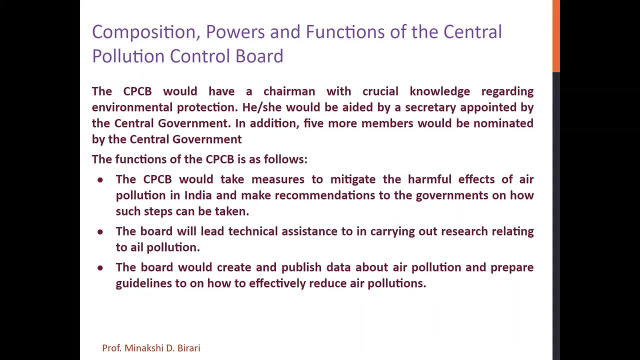 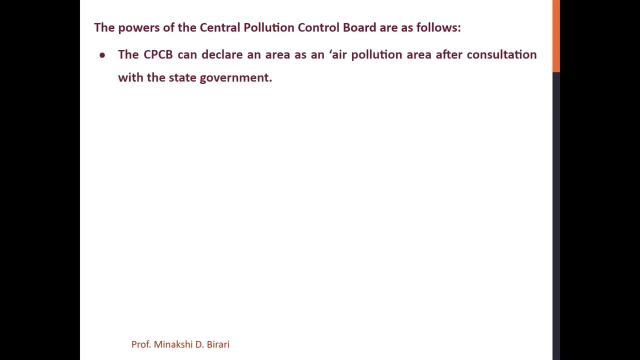 pollution and prepare guidelines to on how to effectively reduce air pollution. so these are the functions of CPCB, that is, Central Pollution Control Board. the powers of Central Pollution Control Board are, as it can declare an area as an air pollution area after consultation with the state government, also the central as well as the state pollution control. 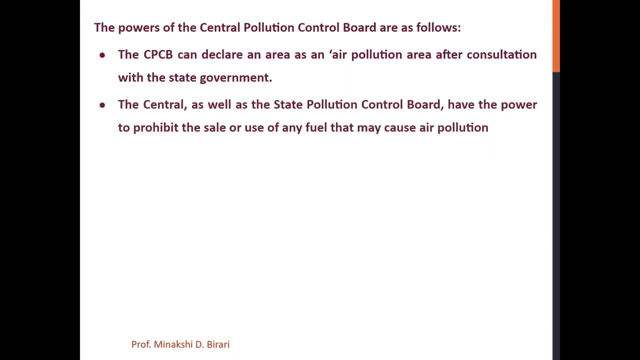 board have the power to prohibit the sale or use of any fuel that may cause air pollution, also having a power to give restrictions for ensuring standards for emission from automobile restrictions on use of certain industrial plants. the Air Act empowers the state and central pollution control ports to carry out. 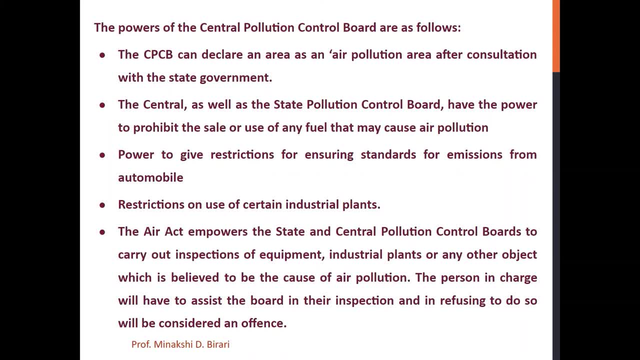 inspections of equipment, industrial plants or any other object which is believed to the to be the cause of air pollution. the person in charge will have to assist the board in their inspection, and in refusing to do so will be considered an offense. so these are the powers of Central Pollution Control Board. 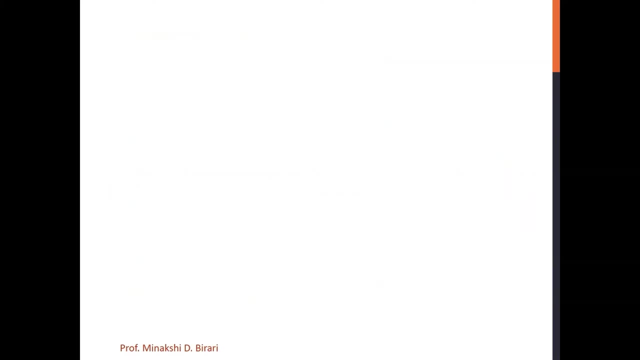 so there are the different air act before 1981 air act first of all, that is, 1948, the factories Act and amendments in 1987, force to express concern for the working environment of the workers. after that, 1981, the air prevention and control of pollution act which are which was 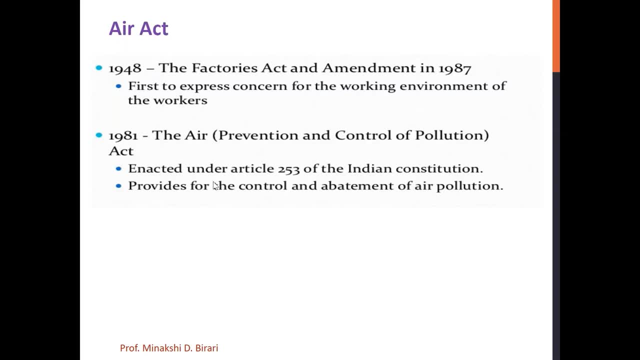 enacted under article 253 of the Indian Constitution, provides for the control and of air pollution. Then, 1982, the Air Prevention and Control of Pollution Rules, which defines the procedures of the meetings of the boards and the powers entrusted to them. After that, 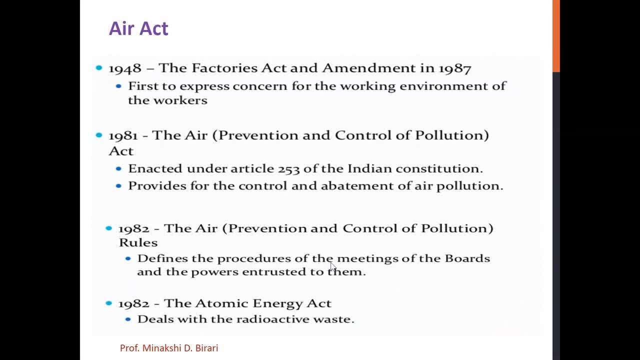 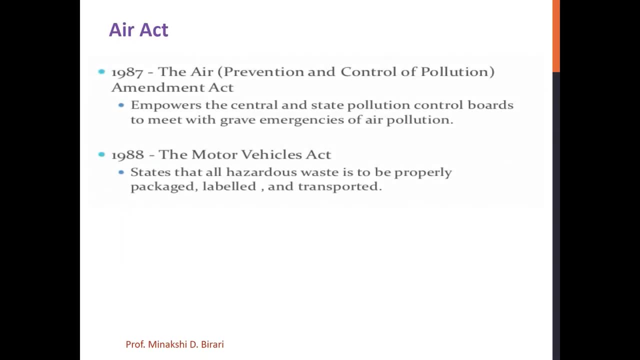 1982, the Atomic Energy Act, which deals with the radioactive waste. Also 1987, the Air Amendment Act which empowers the Central and State Pollution Control Boards to meet with grave emergencies of air pollution. Also 1988, the Motor Vehicles Act, which states: